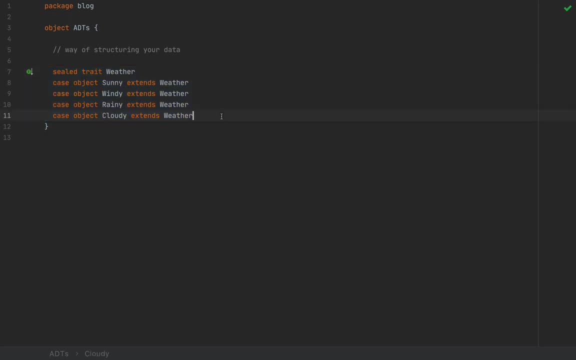 key that looks like this: We've just defined our first algebraic data type, or ADT, And this particular structure, this weather thing, is a so-called sum type. And it's a sum type because a weather, an instance of weather, can either be sunny or windy, or rainy or cloudy, And so 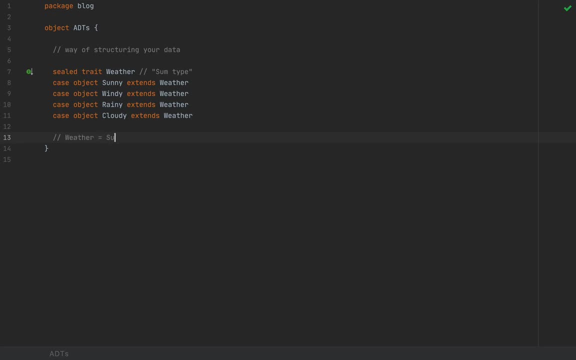 I can say here in the comment that weather is sunny or windy or rainy or cloudy. Now, truth be told, these ors are actually exclusive ors and in Boolean logic they are the same as the plus operator. So this weather type is also called a sum type. 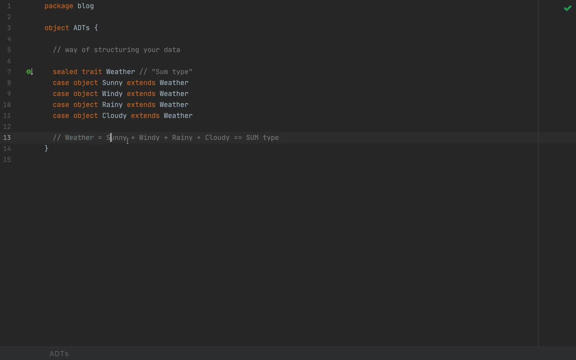 because the big type weather is summed up by the types sunny, windy, rainy and cloudy, which are also the values of their own types, because I've defined them as case objects. So when you have a trait or an abstract type, 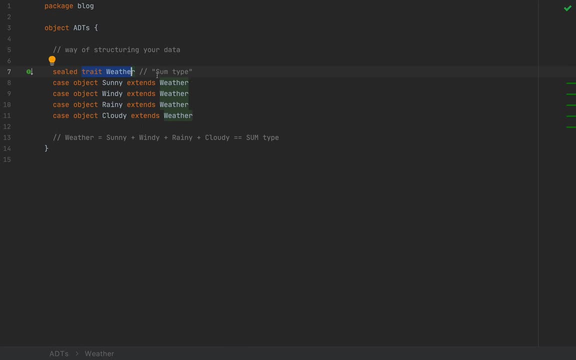 where you lay out all the possible cases. you've just defined a sum type, a sum algebraic data type. Now, in Scala, we usually implement a subtype as a sealed trait or a sealed abstract class, And this helps us with pattern matching in particular, because the compiler can figure. 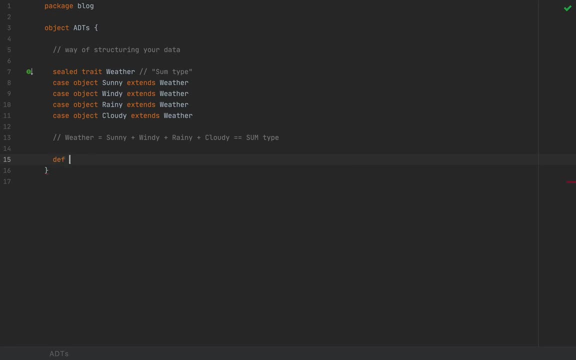 out if we haven't exhausted all the cases. So, for example, if I define a method called feeling which takes a weather instance as an argument and this returns a string, and I'm just going to do pattern match against the weather, so weather match, and I would use case sunny and I would 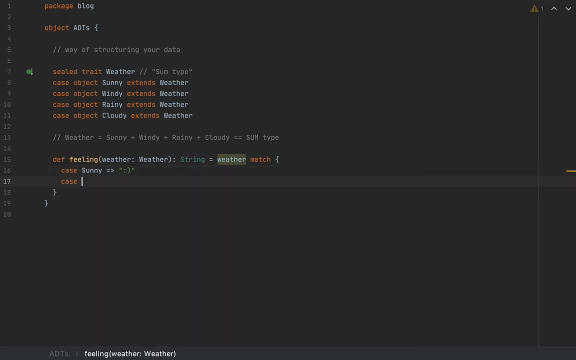 say I would return, for example, this smiley face, and then, if I have a case cloudy, I will return, for example, a straight face, and if I have a case rainy, I would return a sad face. for example, Now, because the weather is a sealed trait, the compiler warns: 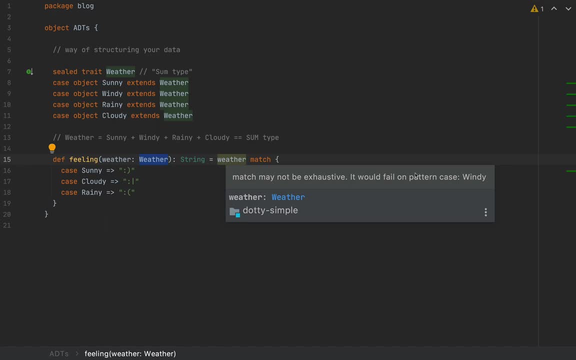 me that the match may not be a sealed trait. So if I have a case cloudy, I would return a sealed class. Now, if I have a case sunny, it would not be exhaustive. It would fail on the pattern that I have not matched against. So this is why we use sealed traits or sealed 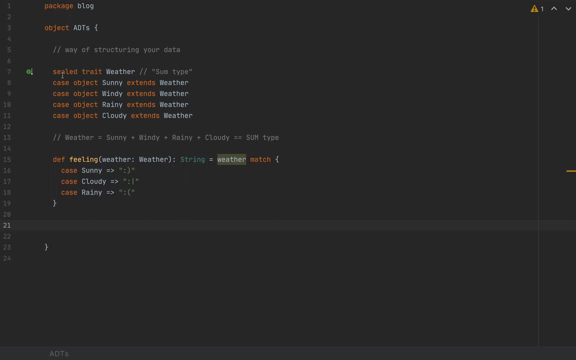 abstract classes. Now for better binary compatibility, you would use a sealed abstract class, because sealed abstract classes cannot be mixed together, And on the same token, we use case objects here for the various options that we have, because case objects give us a set of useful 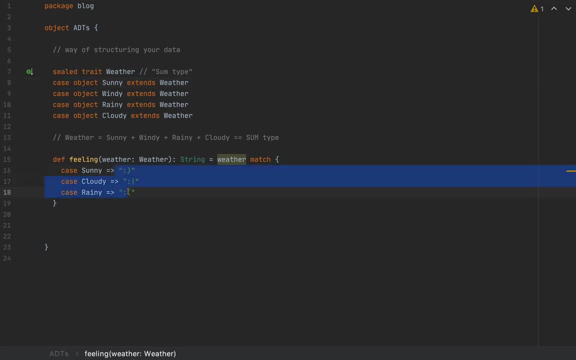 features, For example, the unapply method allowing us to use them in pattern matching. We have free implementations of equals and hash codes and the extension of serializable, so we can send these values over the network. So we've discussed about a sum algebraic data type. I'm now going to discuss 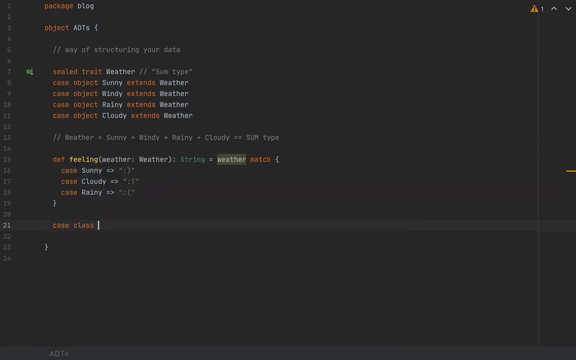 about a product type and I'm going to define a case class and I'm going to name this weather forecast request. This is something that we would send to a web service that would give us some data related to weather forecasts and, for example, I would like to pass some latitude and longitude. 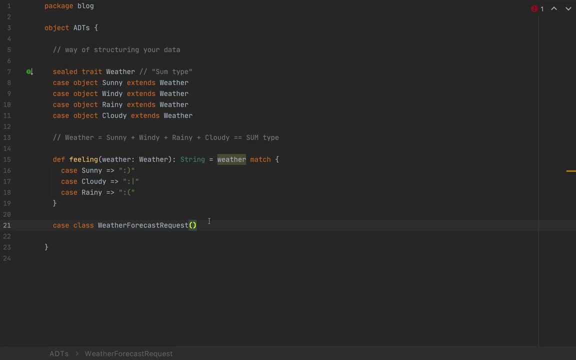 of the place where I would like the weather forecast. So I'm going to say latitude as a double and longitude as a double. All right now. this case class also defines its constructor. So if you know the Scala basics, when you define a class and you pass in some arguments, then you 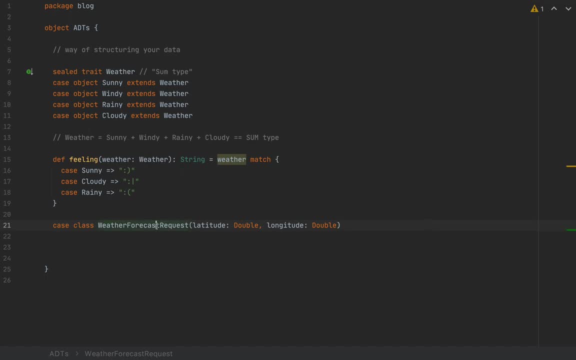 also define its primary constructor. So, in order to instantiate one of these weather forecast requests, you would need to pass a latitude and longitude. Now, in the language of types, this is equivalent to a function, that is of the form double and double, and then you would. 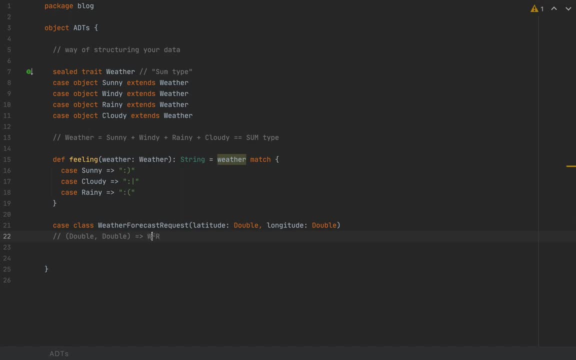 return a weather forecast request, abbreviated WFR for short. And so for every pair latitude and longitude you can define a weather forecast request, And so the weather forecast request type WFR is essentially a Cartesian product between double and double, because for every pair you can 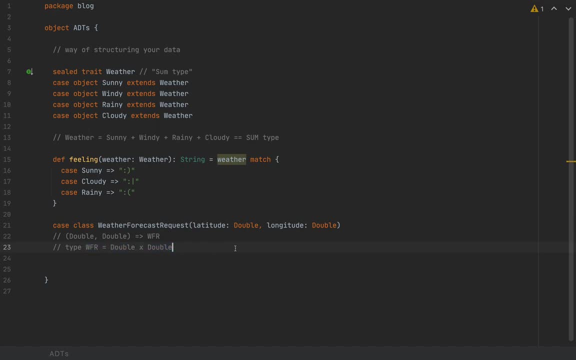 define a weather forecast request. Now, this Cartesian product type is called an algebraic product data type, And product types are usually implemented in Scala as case classes. So when you define your data models, you should use case classes. Now, case classes, as you're probably 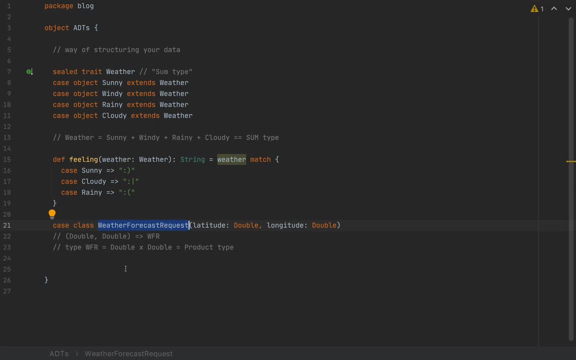 aware, have a lot of features baked in, For example, companions with apply methods. You have the serial usability, which you also saw in objects. You have equals and hash codes and to string already for you and a bunch of other features. So case classes are a really powerful tool for this. So the type 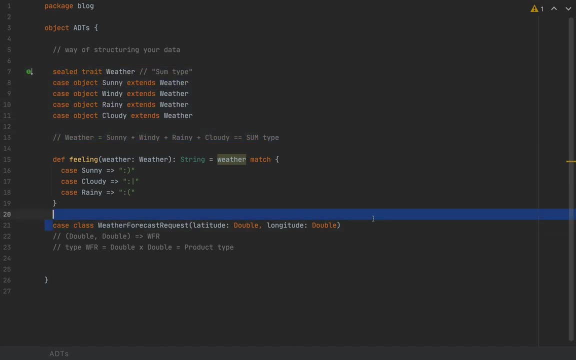 representing a weather is a sum type and the type representing a request to our weather forecast server is a product type. There's also a mixture of those and we call those hybrid types And because we have a hybrid type, we will have a sum of various product types. So I'm going to define hybrid types. 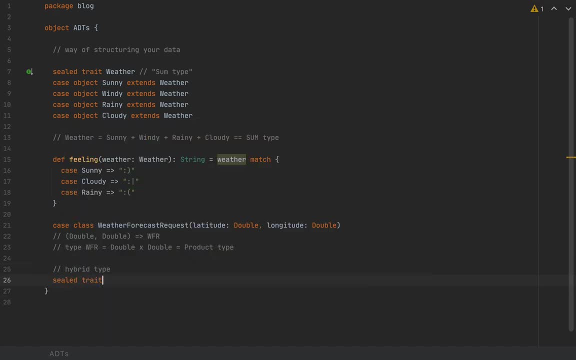 For example, I'm going to use a sealed trait and I'm going to define the response type that our weather forecast server will give back to us. I'm going to call this forecast response, or let's call this weather forecast response. Now, this is the trait. Now, let's say that this server gives back. 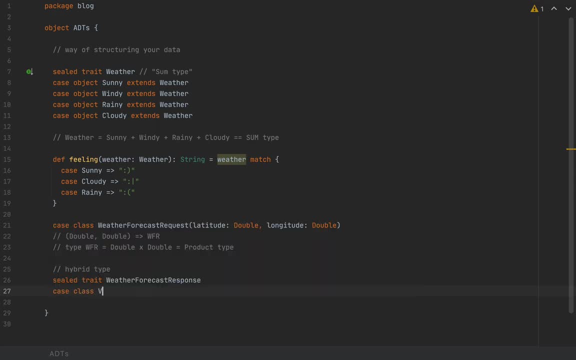 two kinds of answers to us. I'm going to define a case class- Let's call this a valid- and I'm going to contain a weather inside, So I'm going to use weather inside. So the 받. I'm going to write weather here and it extends weather forecast response. So this is the valid. 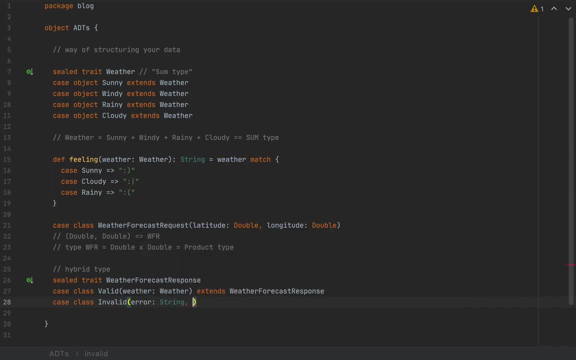 response and I'm going to also define a case class for invalid and I'm going to wrap, for example, an error as a string and the description of that error or the reasoning behind it. as a string- and this also extends weather- is a sum type, But each of the possible cases is a product type And same for the other. So we have. 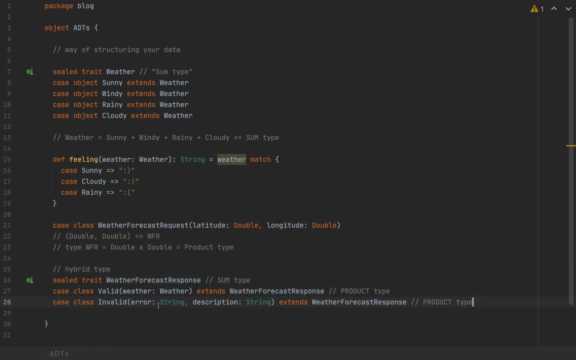 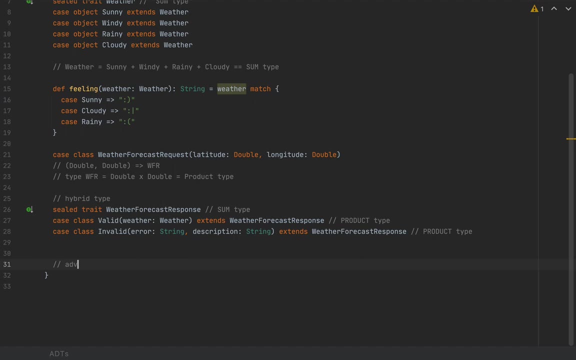 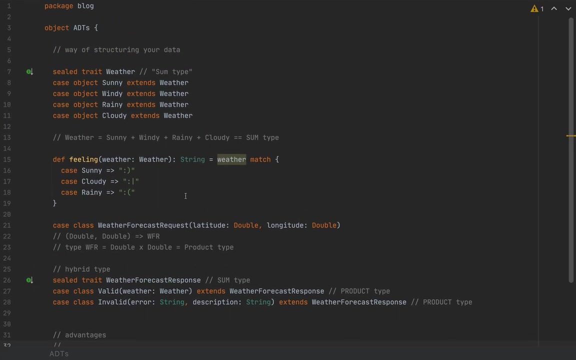 basically a sum of product types which is a hybrid type. So we've discussed about the main types of algebraic data types, But what are the main advantages there? And I'm going to mention a few. First of all, and probably one of the most important advantage of algebraic data types and of 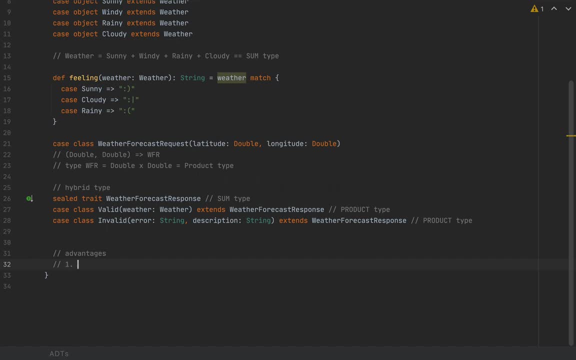 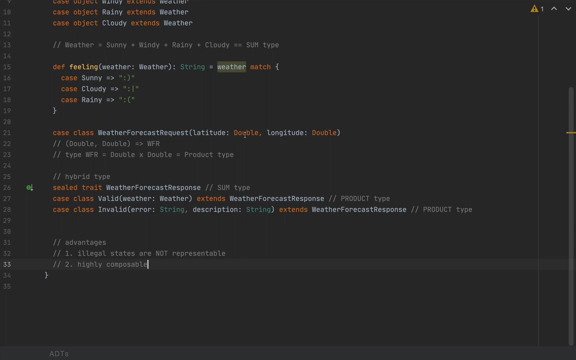 this style of structuring your data is that illegal states are not representable, And I'm going to exemplify what I mean by that a little bit later. The second advantage is that ADTs are highly composable, That is, we can use ADTs within other ADTs And, just to give an example, this hybrid. 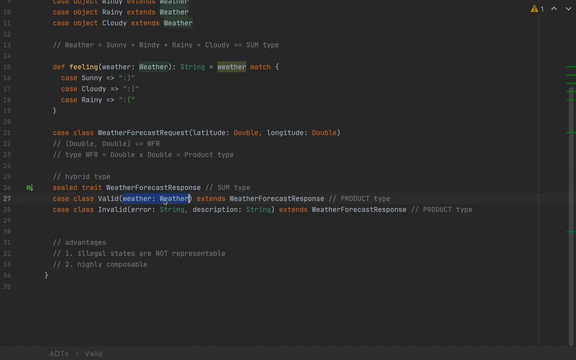 type is a product type, So we can use ADTs within other ADTs And just to give an example, this is a perfect example because the weather, which is also an ADT, was used in one of the cases for the weather forecast response. So they can highly compose with each other. The third advantage is 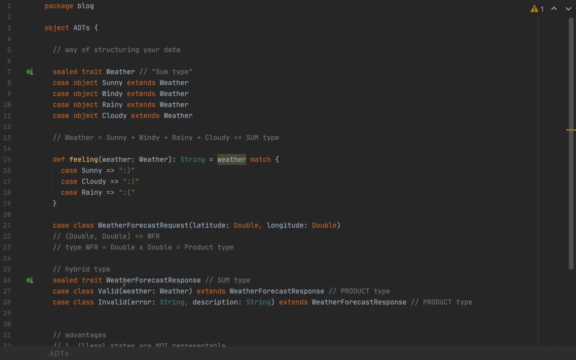 that ADTs usually store only data, That is, they store the arguments with which they are constructed or they themselves are the values of the potential data structure. So they contain just data, not functionality, And this composed with the principle of functional probability, which is the principle of functional probability, which is the principle of 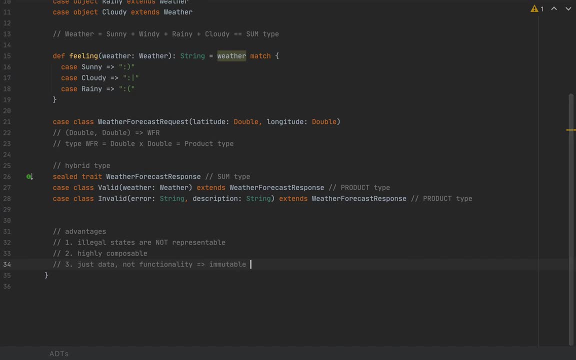 programming. This leads to immutable data structures And all the advantages that come with that. For example, it's very, very easy to track which value came from where in our code with immutable data structures. This comes from experience And also advantages related to. 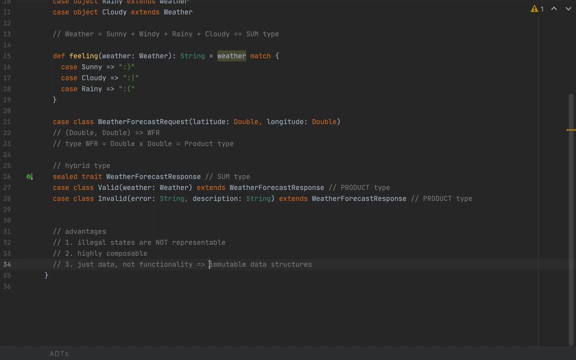 parallel and distributed applications. because no thread can mutate a data structure, it will have to create a new one. In fact, I'd go as far as to say that this should be an advantage of its own. So this should deserve its own bullet point. And because of the fact that ADTs are just data and 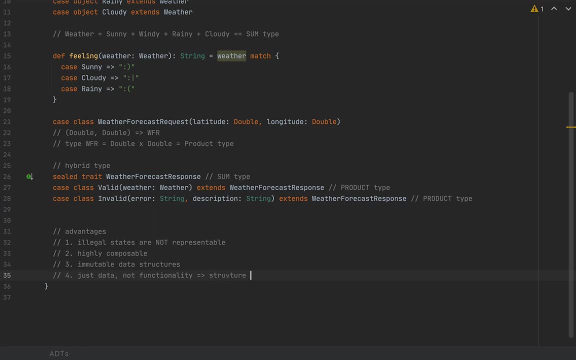 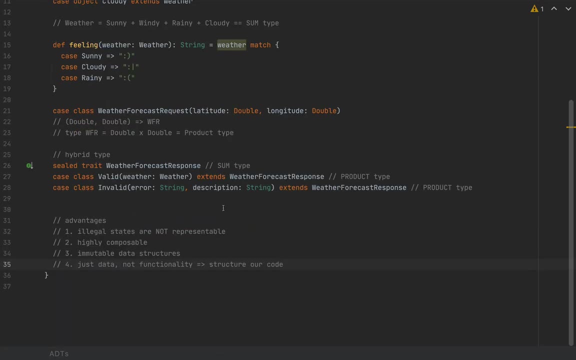 not functionality. this makes it easier for us to structure our code in general And make it easier for us to publish libraries and data type definitions. Now, I mentioned a minute ago that illegal estates are not representable. This is one of the major. 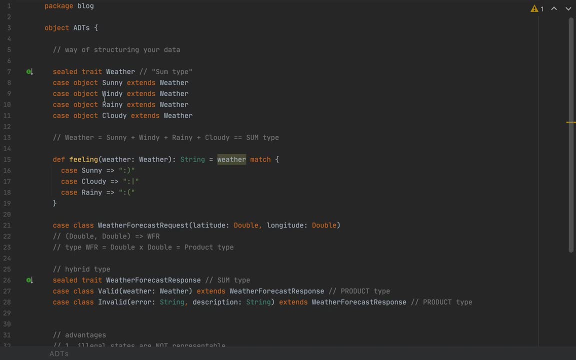 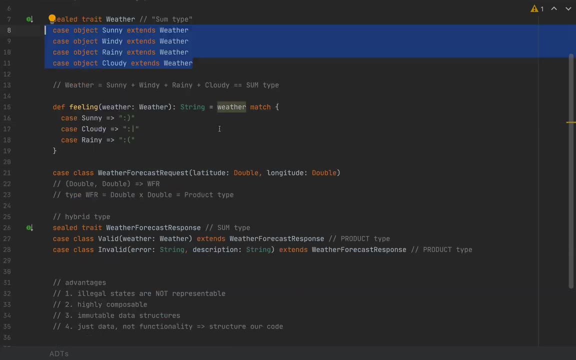 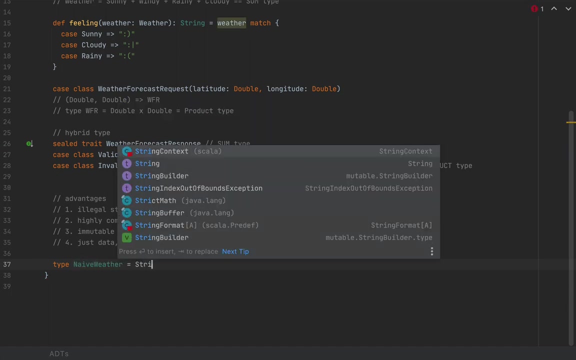 advantages of ADTs. What do I mean by that? Let's go back to our weather trait. Instead of the weather trait, and with all these case objects, we could have said something like type, let's call this naive weather, which is a string, And instead of using that weather type we should have used or we could have. 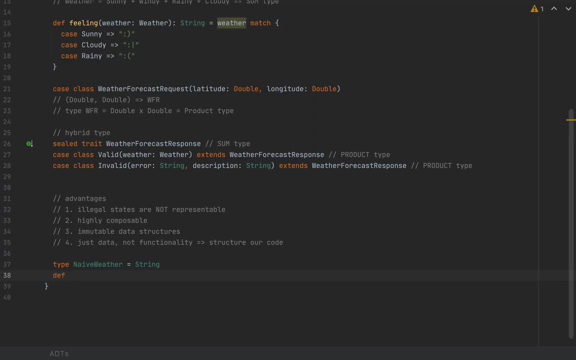 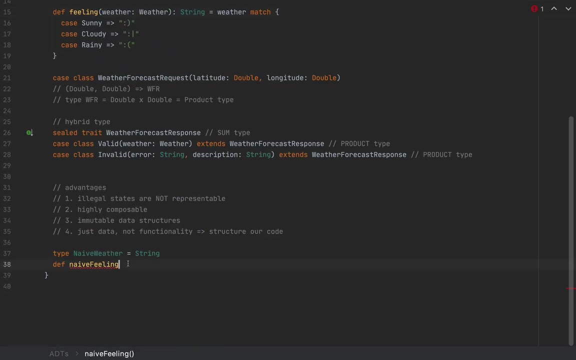 used a string And, for example, we could have said: let's call this naive feeling. If you remember this feeling method that gets a weather as an argument, naive feeling could have had a weather as a string And there you would have weather match. 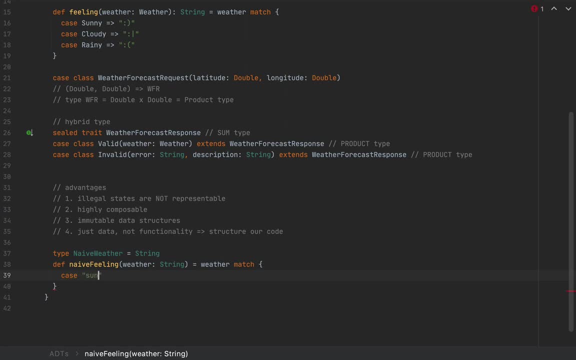 And then you have case sunny, And then you would put on that smiley face and so on and so on. So here you would have some other cases. Now what would happen if you do naive feeling and then you pass in the string, let's say 45 degrees. What do you do then? Most likely, your application doesn't. 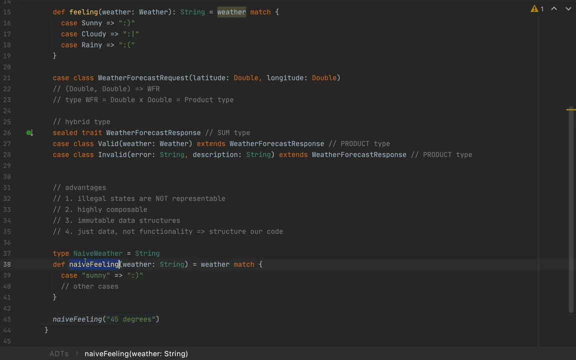 support this kind of string, And so this method would fail with a match, And so you would have to dochi match, so you would have to do match error. But this is a very, very easy case if you have a large code base with lots of states. 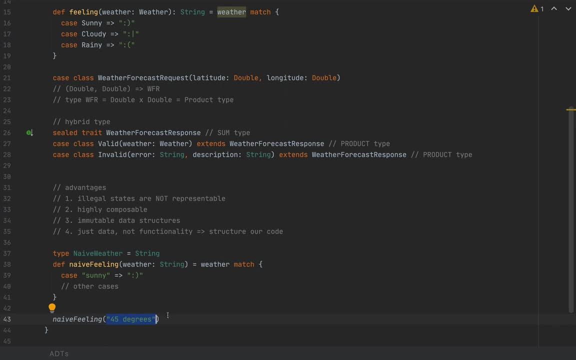 that you do not account for. this kind of invalid argument will crash your entire application, and you don't want that, And so you want to limit the kind of values that you accept here in this method, And so instead of a string, which is a very loose kind of data, you use this Siegel trade. 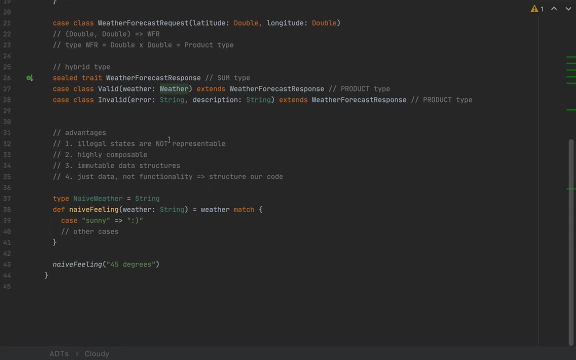 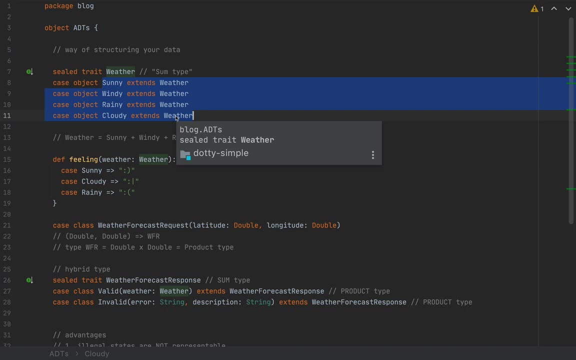 and then you explicitly allow, and then you explicitly allow these options to handle in your application not representable, because with this kind of seal trait and this hierarchy you would not be able to pass anything else than sunny, windy, rainy or cloudy. This is the big argument of making 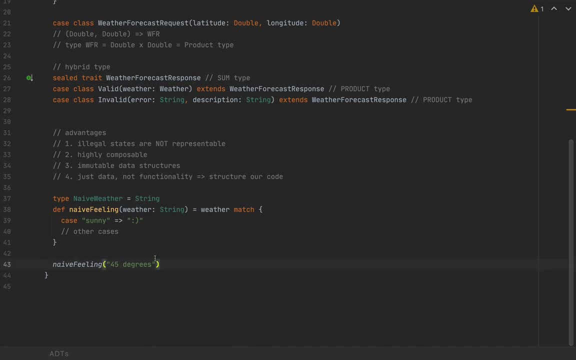 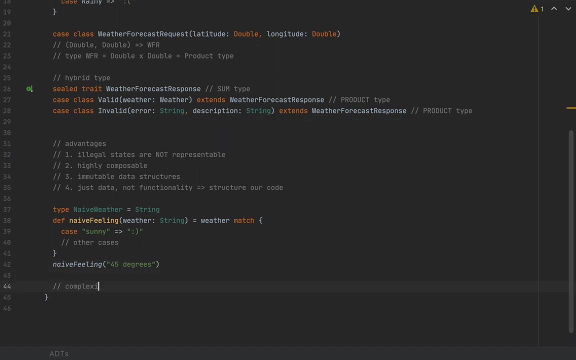 illegal states unrepresentable. There's also a soft argument for reducing the complexity of an ADT. What do I mean by that? The complexity of an ADT is the number of possible values of that ADT. Now our goal while designing an application for the real world and modeling our 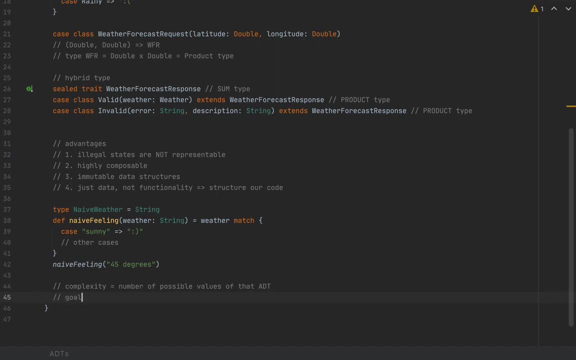 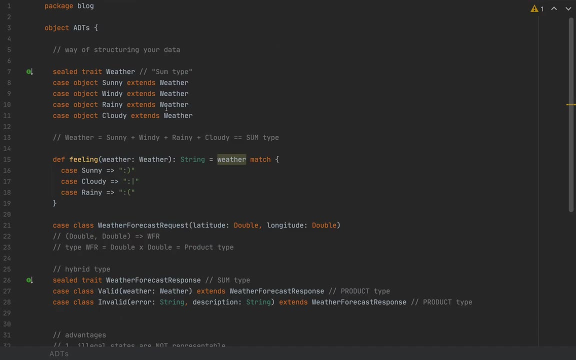 data, for the business logic that we want to implement is to reduce this complexity. And how can we reduce the complexity? Well, one way of reducing the complexity of the weather type would be to explicitly allow for the possible values that you might want to support, So not.